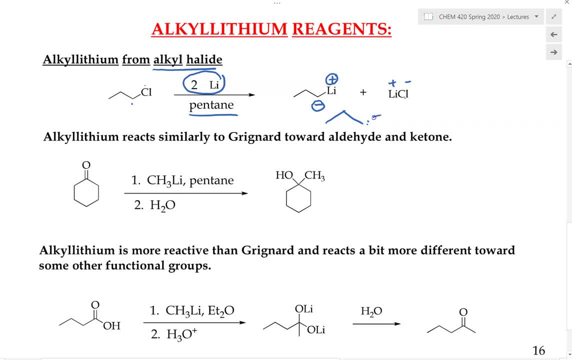 carbon, And so what this would do is that it would give one electron to one chlorine and give all the electron to one lithium, And we can also abbreviate this as follow: Or we can draw the covalent bond between the carbon and the lithium. 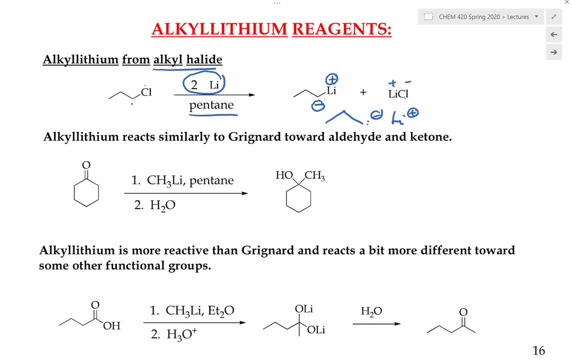 Now. so let's now go over the chemical reactivity of the alkyl lithium reagent. So they behave similarly to the Grignard reagent towards the aldehyde and the ketone functional group. So if we would have aldehyde and ketone and react on this with our, in this case, methyl, 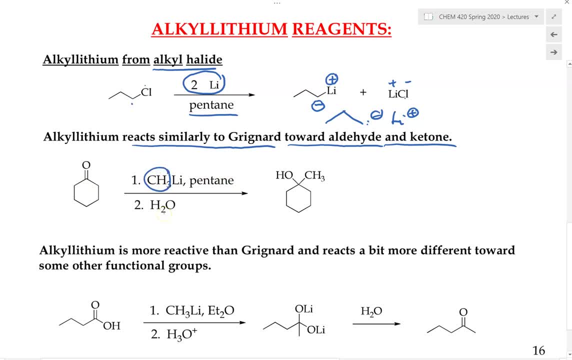 lithium reagent. in the presence of pentane, followed by water workup, we'll be able to convert this into the tertiary alcohol. So this reagent- right here it also is very, very nucleophilic And in fact it is even more nucleophilic compared to the Grignard reagent. With this come in. 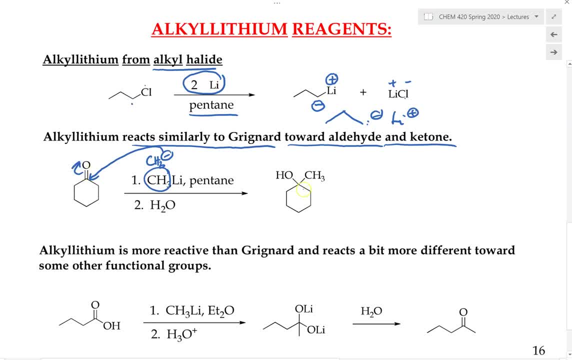 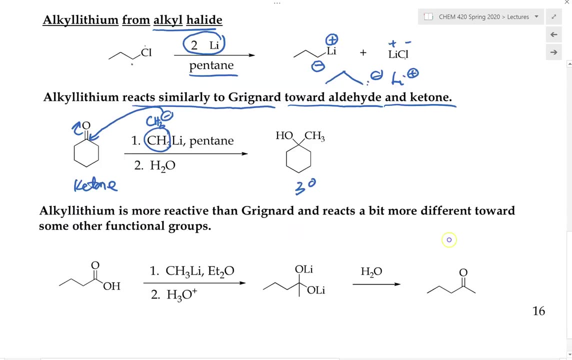 I cut that and kick that off and followed by the protonation step to protonate our alkoxide and we'll be able to produce our tertiary, tertiary alcohol, In the case that we start out with a ketone. Now, why are the alkyl lithium reagent more reactive than the Grignard reagent? And again, 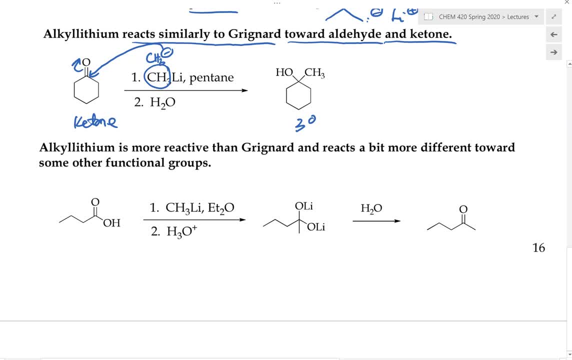 this is something very important for us to remember and understand. The alkyl lithium reagent is even more reactive than the Grignard reagent And therefore they behave slightly different to some other functional group. in comparison to the Grignard reagent, For an 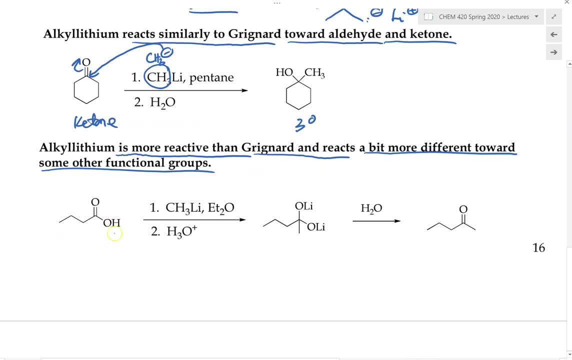 example, we have seen that when we take a carboxylic acid and react it with the Grignard reagent, it will undergo acid and base reaction, but not the nucleophilic addition reaction. However, if we were to use the lithium reagent instead of the Grignard, they now will be able. 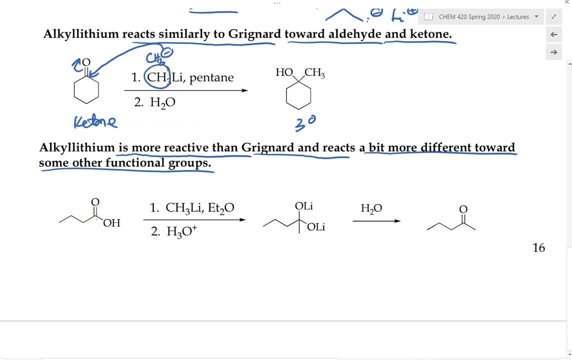 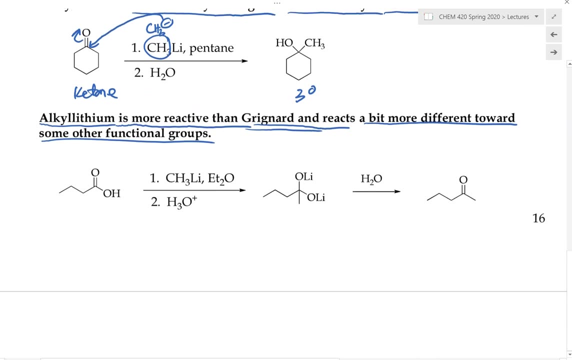 to do nucleophilic addition to this carbonyl carbon right here. So that is one very, very important and distinct differences between the reactivity of the alkyl lithium reagent versus the Grignard reagent. Let's now discuss why the alkyl lithium reagent is so reactive and even more. 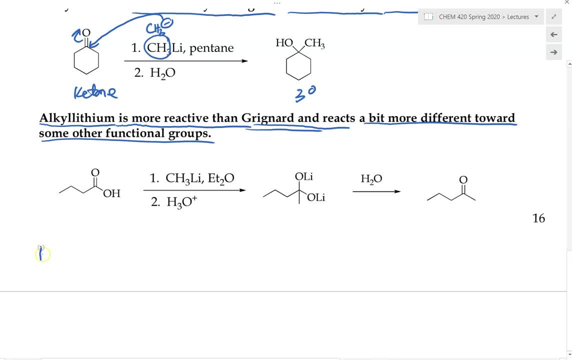 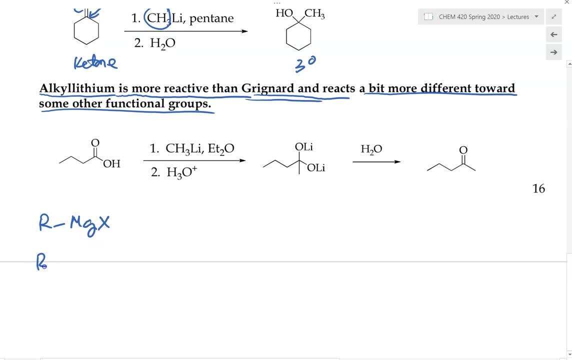 reactive than the Grignard reagent. When we have our Grignard reagent, we will be having this bonded to the magnesium and the halite, versus in comparison, this would then be our lithium reagent. And now notice the following, the charges: this magnesium- right here, E two. this x- right here is E two. also one here, Ba 2 and B 2.. 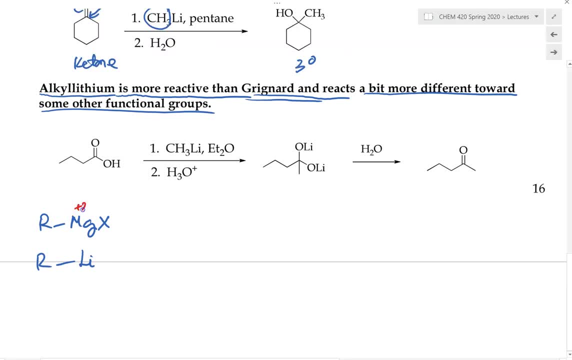 When I will connect these two Aíabaeûs with an Alkyl lithium reaction. So now the bitterness on the performant. let's perform some review with our Dr Allen Lieberman. Let's not worry about the느� strategy here, because I have very good conscienzails here. There's more approach as to why it works. 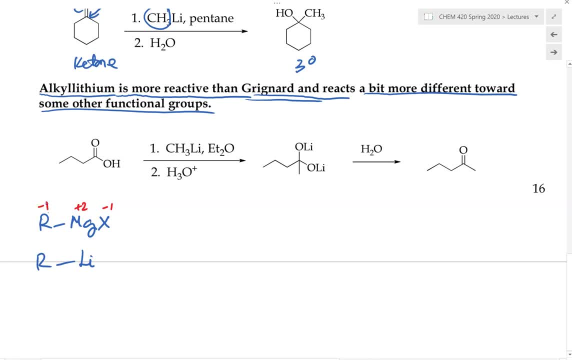 This X right here is negative 1, and therefore this carbenion right here is negative 1.. In the case of the alkyl lithium reagent, this is plus 1, and this is negative 1.. So in both cases, then, the bond of the charges of the carbenion are both negative. 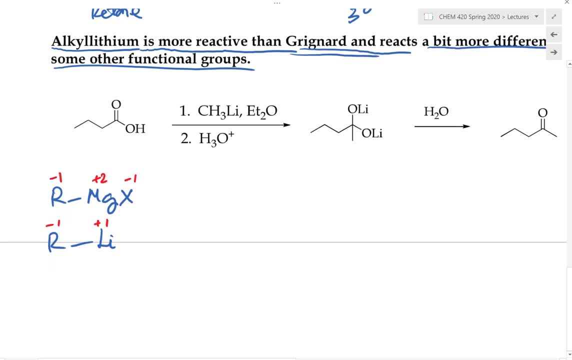 But there's some differences, and in fact some very important differences, between the two of them. First of all, the ionic bond between the ore of carbenion and the magnesium, in the case of this Grignard reagent, is actually stronger compared to the bond between the carbenion and the lithium. 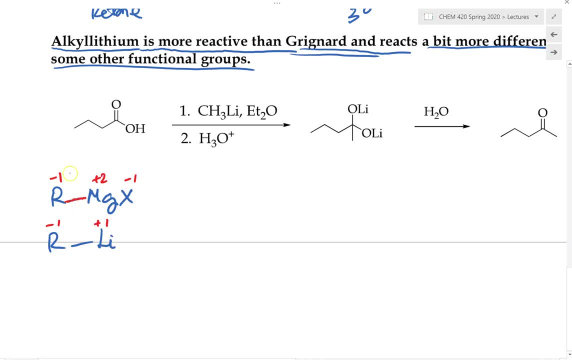 And the reason why this bond right here is an ionic bond And right now we have the attraction between something negative 1 and something positive 2.. So this bond right here is strong Versus the bond in the case of the alkyl lithium. 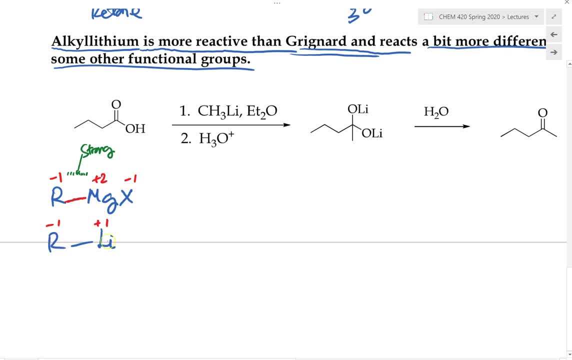 So this carbenion right here is negative 1, and the lithium is positive 2. So they are attracted to each other ionically as well. However, this is then a weaker ionic bond, And because this is a weaker ionic bond, this can be broken easily. 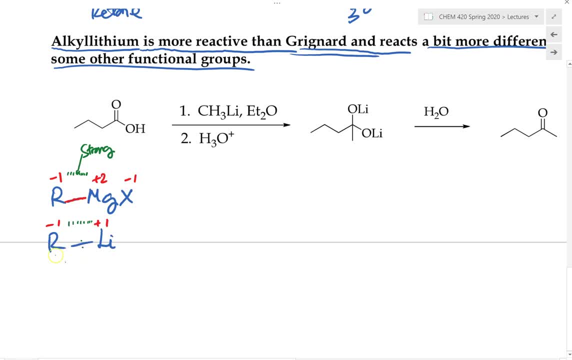 And therefore we can see that the electron can then go to this alkyl carbenion right here more easily And therefore it's more readily available to react. And again it is due to the fact that this ionic bond right here is weaker. 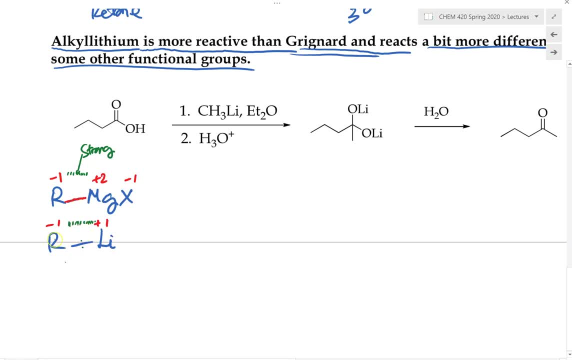 Because it's weaker. it tends to dissociate further, making the charge on this carbenion become more negative And therefore more reactive. So we can see this is more reactive because it tends to be more negative, So the ionic bond to the carbenion is weak. 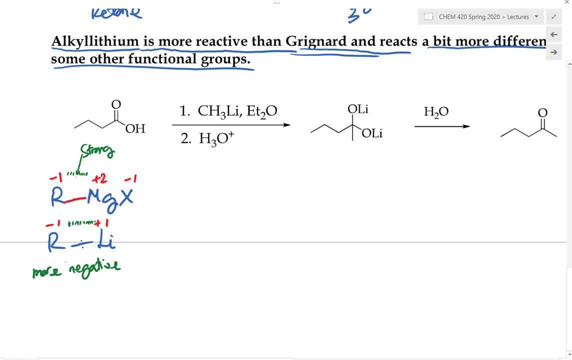 Versus here. this bond right here is stronger. So that's important for us to understand why the alkyl lithium reagent are more reactive than the alkyl, than the Grignard reagent, As a nucleophile and also as a base. 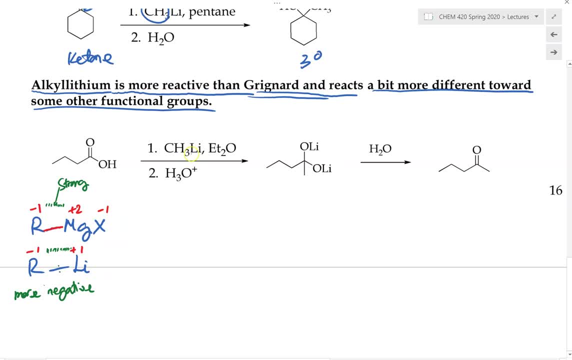 So now let's go over the chemical reactivity of the alkyl lithium reagent with the carboxylic acid. So first, when we take this, then we know that the carboxylic acid has this proton right here that is acidic. 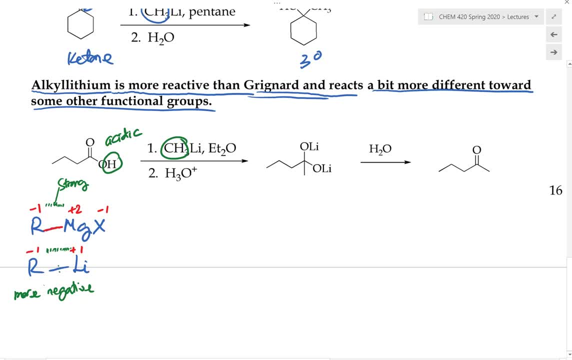 So if we were to be taking treatment this with the alkyl lithium reagent, this reagent can also behave as a base and as a nucleophile. Anytime acid and base reaction can happen, then it will happen Before nucleophilic addition reaction. 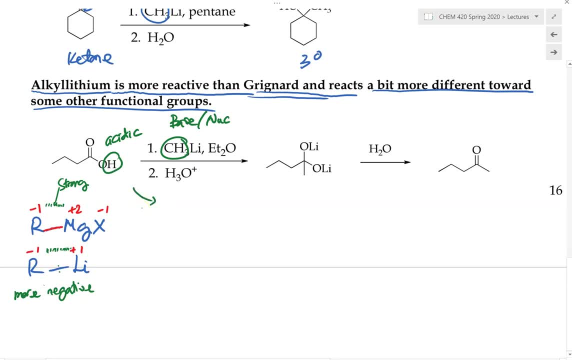 So therefore, the first equivalent of what we will see is that it will undergo acid and base reaction first. With this coming, pick up this proton, give an electron to this oxygen right here, So first we will be able to produce this carboxylate. 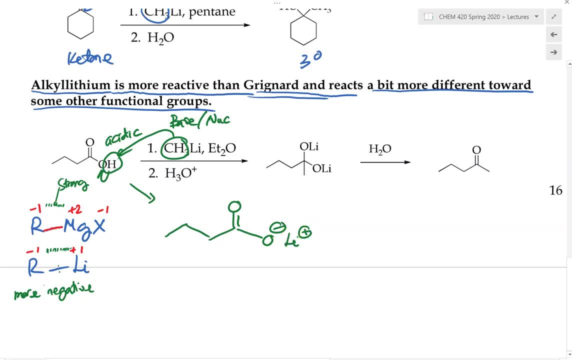 And now one of the lithium will be binding to this oxygen as the counter ion. Now here is what happened right here. If we were to have excess of this reagent right here, the excess reagent will be able to come in and add on to this carbonyl carbon, right here. 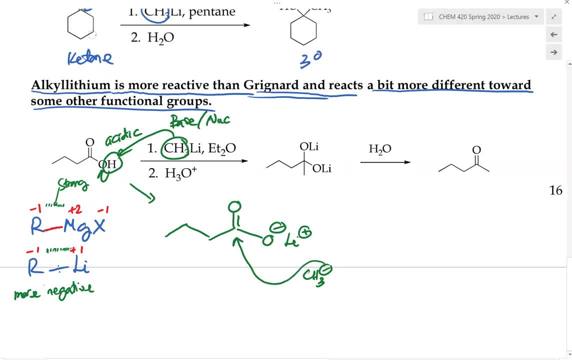 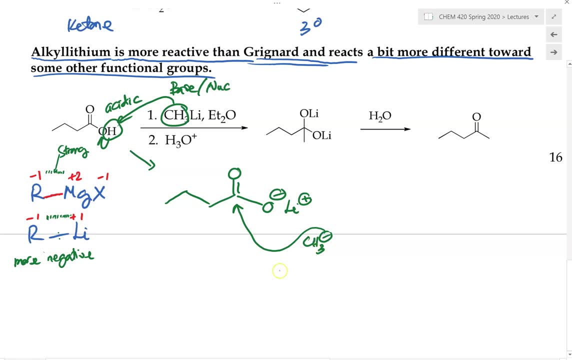 And this is very, very different in what we have seen from the Grignard reagent, The gray reagent from Grignard. if we were to do the Grignard reagent, this carbenion would not be able to come in and attack this carbonyl carbon. 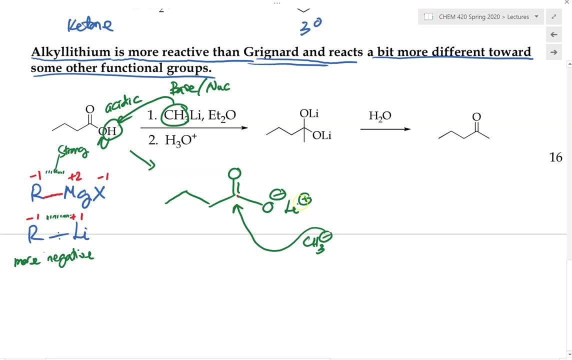 Versus if we were to use the alkyl lithium reagent now, this carbenion would be able to come in and attack this carbonyl carbon. So why? The reason why is as follows: It is due to the chemical reactivity of this carbonyl carbon right here. 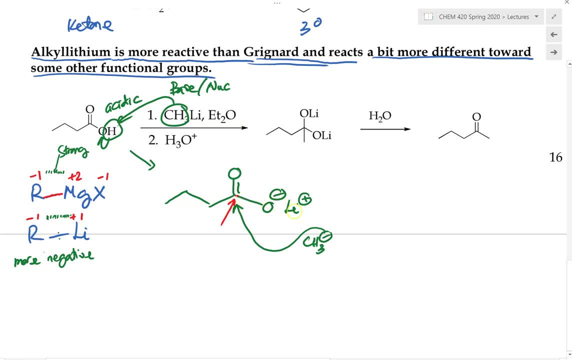 In the case that this carbonyl carbon right here is bonded to the lithium, this bond right here between the lithium and the oxygen. this is actually a very strong bond right here, And the reason why is because Both oxygen and lithium are on the second row elements. so they are quite similar in size because they both belong on the second row, clearly not in the same size, but then they belong to the same row on the periodic table. so therefore they are similar in size. 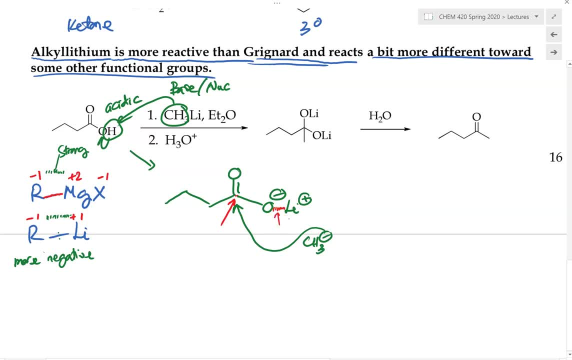 And the strength of this ionic bond right here is then dependent on size, and therefore this is quite a strong bond, And the stronger this bond is, the more this part of lithium will be able to neutralize the negative charge. And the stronger this bond is, the more this part of lithium will be able to neutralize the negative charge on this oxygen right here. 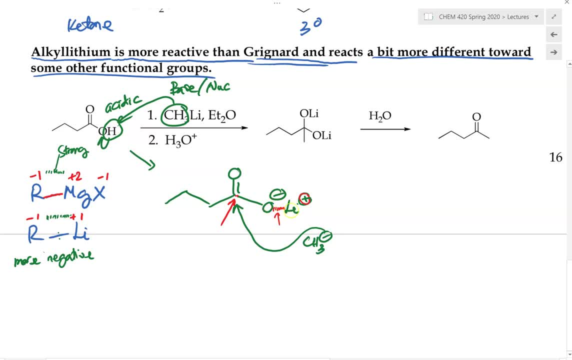 And as this oxygen right here is becoming neutralized due to the strong bond to the lithium, it will not be able to donate as much electron to form resonance to the carbonyl carbon. So in this case, right here, this lithium is effectively taking the electron away from this negative oxygen right here, reducing the positive power charge on reducing the ability of this oxygen to donate electron to this carbonyl carbon. 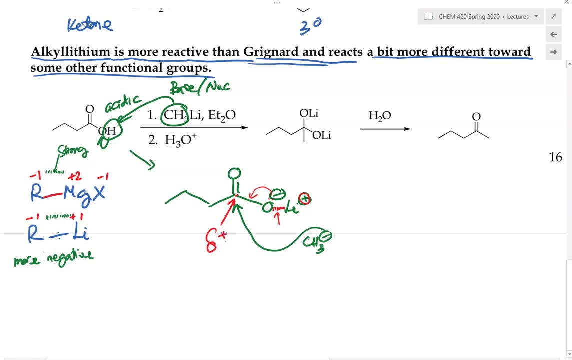 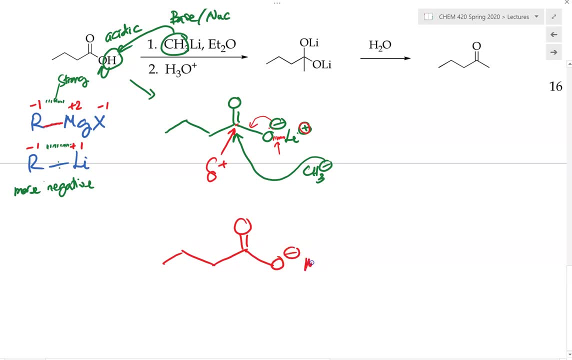 So therefore this carbonyl carbon right here becomes more partially positive compared to the counterpart where we would now be having the Grignard reagent, In this case right here. so this positive charge right here it is not as big compared to this positive power charge in the case of this reagent involving the lithium. 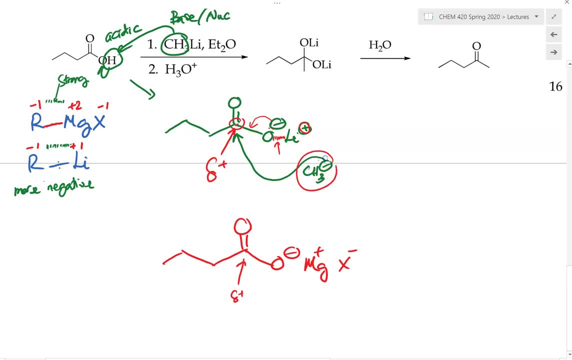 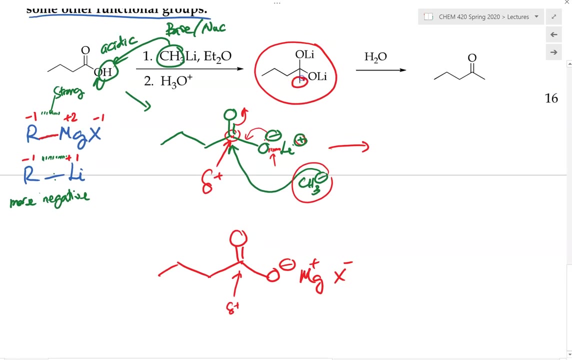 And therefore the carbon ion will be able to do another addition to this: carbonyl carbon right here will come in, can attack that and kick this off. so in the product we will be having this And again, this is the methyl group that comes from the reagent producing this salt right here. so this, basically, is the bis-lithium salt. 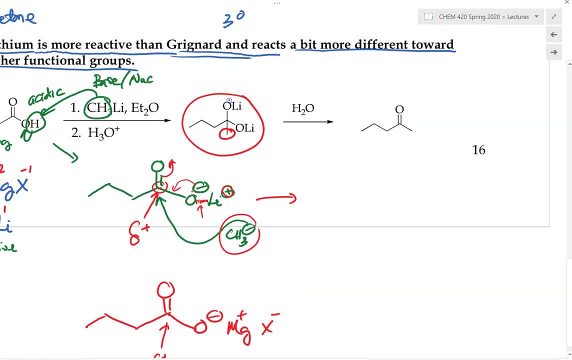 And, following the water workup step, then both of this will be able to come in and pick up the proton from water and initially we will be having this product right here And this is called an acetal, and acetal in the presence of water it will break up and kick off this and this can pick up a proton from water again. 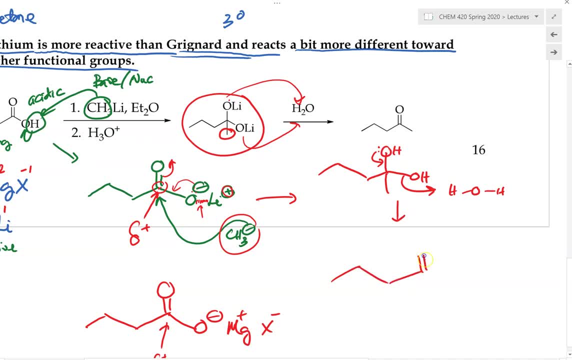 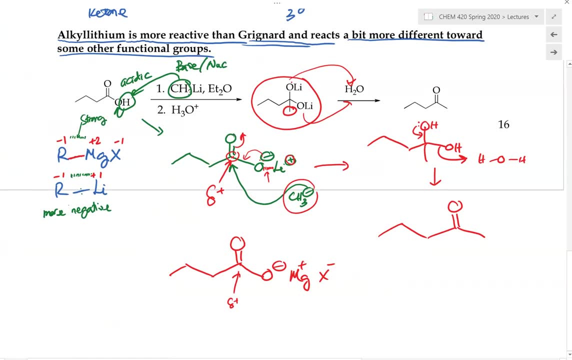 They are not very stable so they will be breaking up to produce lipomon and convert this into a ketone. So alkyl lithium reagent reacts with the carboxylic acid to convert the carboxylic acid into the ketone. 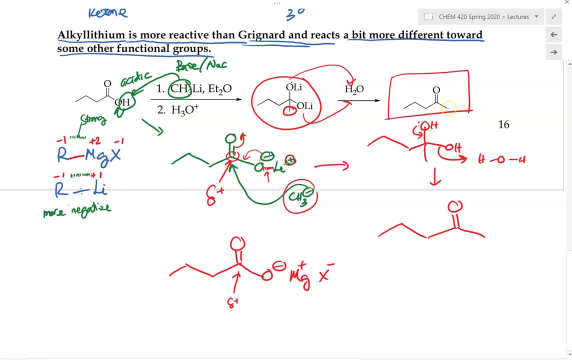 And on this ketone right here, one of this alkyl group. from this ketone right here, it comes from the alkyl group from the alkyl lithium reagent. so please remember that, so that way we can draw the product quickly. 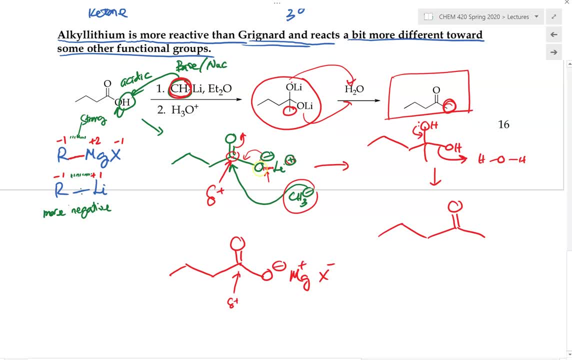 Versus if we were to treat this, the carboxylic acid, with the grignard reagent, we will only be able to do acid and base reaction. So that's one of the very big differences between the reactivity of the carboxylic acid and the carboxylic acid. 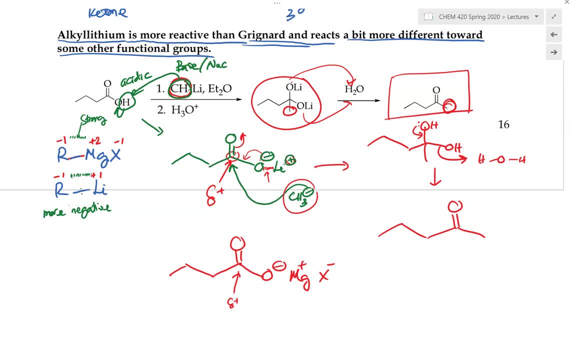 So that's one of the very big differences between the reactivity of the carboxylic acid and the carboxylic acid. So this is the reaction on both the alkyl- and the grignard reagents. So this is the reaction on both the alkyl- and the grignard reagents. 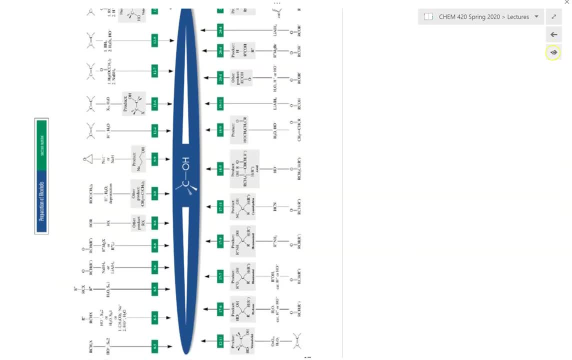 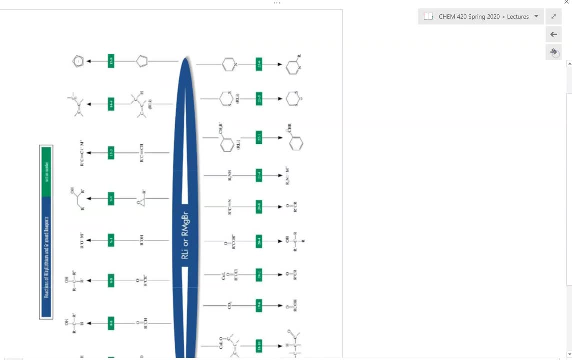 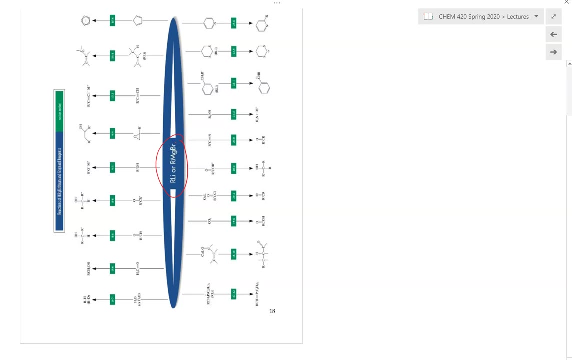 On this next slide right here. then this can basically go over the chemical reactivity. this is a reaction map right here of how we can make the alcohol. This following table right here shows the reactivity of the lithium, alkyl lithium and grignard reagents in terms of how they react with the other functional groups. 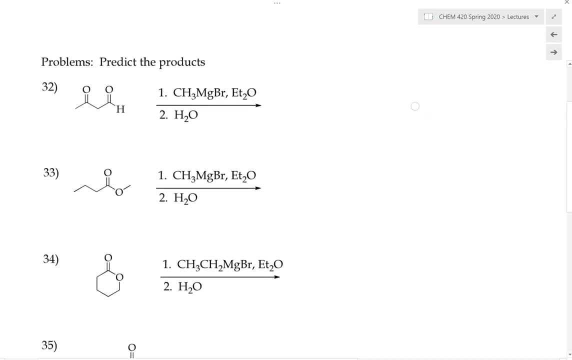 And now lets try how we can do this. a few practice problems involved in this reaction right here. So let's first try number 32.. So in this 32 right here, when we take this a substrate, reacting this with the Grignard Reagent, in which 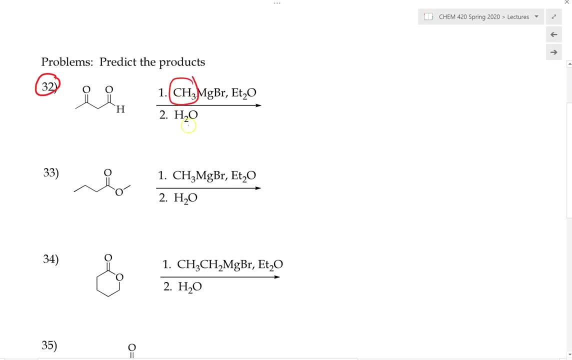 the cardanidine is a methyl group followed by the water workup as a separate step, what would be the product. So we can see here, in this case, right here, we both have an aldehyde and a ketone right here and both of these are good electrophilic, have good electrophilic carbonyl. 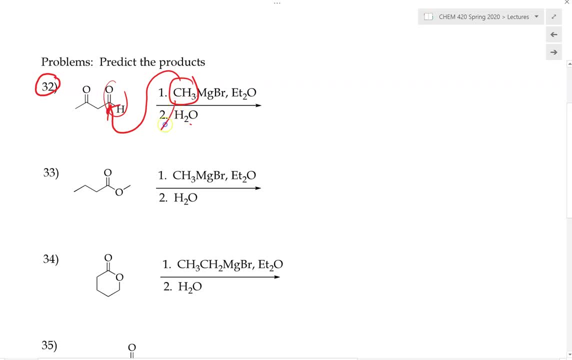 carbons, so therefore they can be attacked by the Grignard Reagent And converting the ketone now into the alcohol. and now we have a methyl group and this methyl group right here comes from the Grignard Reagent. And, as for all the aldehyde, now be able to add another methyl group right here. 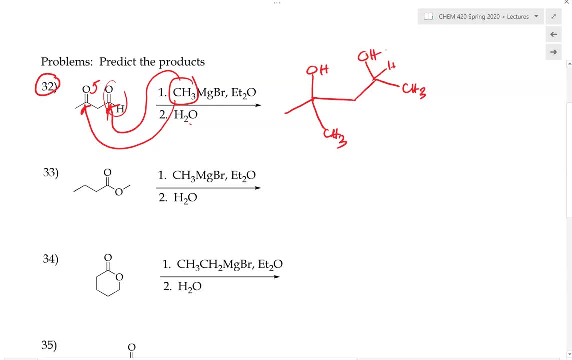 and this then changes. It is changing into the prime, in this case right here, this changing into the second alcohol. so this is a toshino alcohol right here and this is a second alcohol, and that will be the structure of the product.